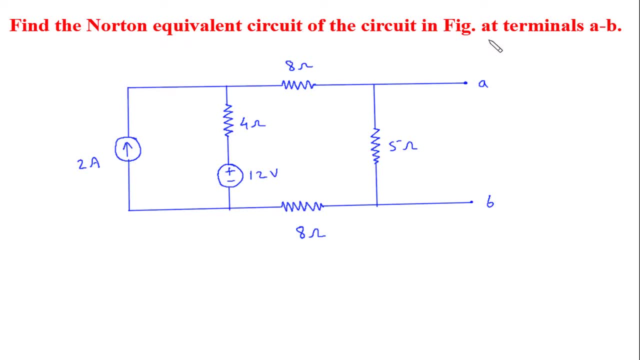 Find the Norton equivalent circuit of the circuit in figure at terminals a, b Solution: First of all we will redraw the circuit. Now we have to find i n and r n. So to find first, we will find r n. 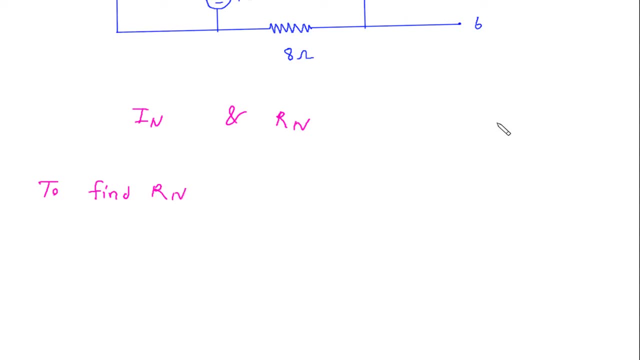 To find r? n, turn off all independent sources. So this is the current source, so this will be open circuit. This is the voltage source, so this will be short circuited And this will be r? n. Now, as we can see that 8 ohm, 4 ohm and 8. 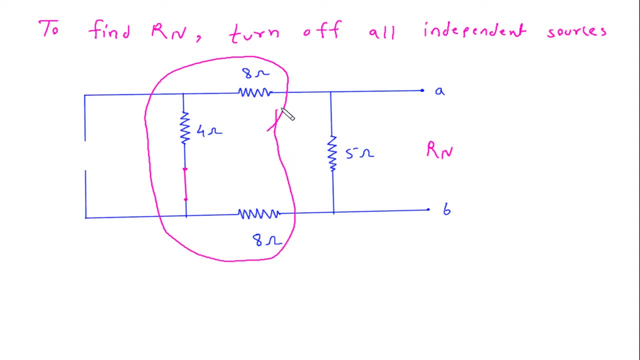 ohm are in series, So this will be 20 ohm. Now this 20 ohm parallel with 5 ohm, So this will be 20 into 5 by 20 plus 5.. So this will be 4, 4 ohm. 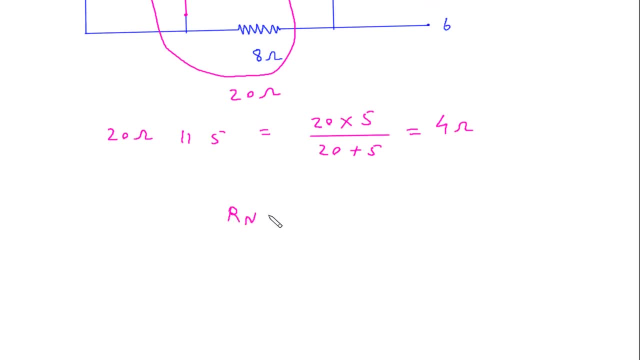 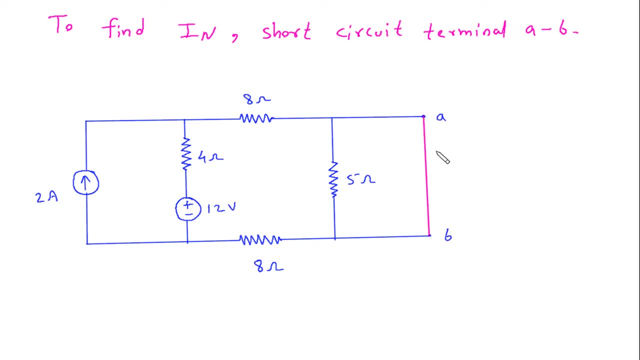 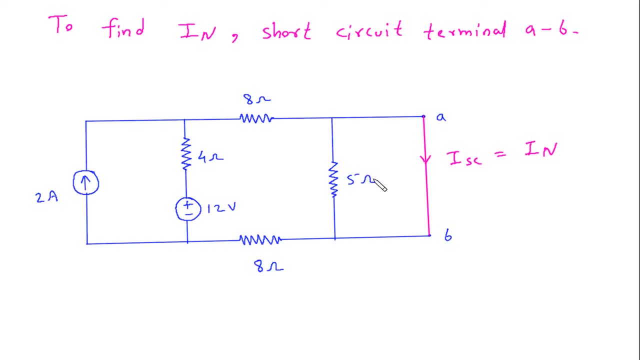 Now, as you can see that this 5 ohm resistance is short-circuited, So this will be 0.. So let's say, this is loop number 1 with current i1 and this is loop number 2 with current i2.. 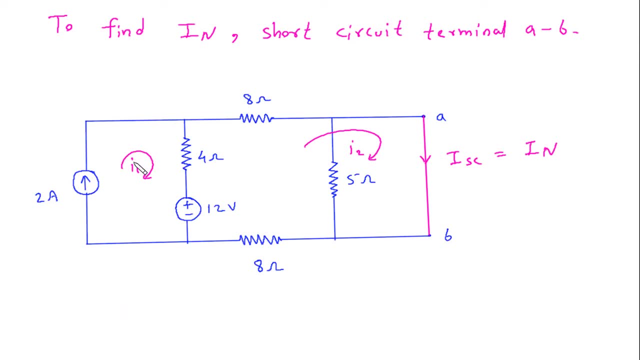 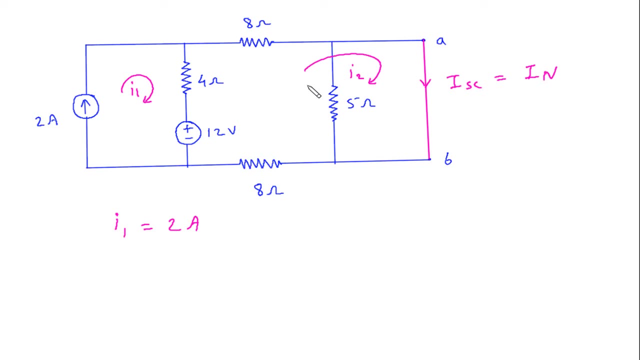 So apply before that. we can see that I1 is equal to 2A. Now we will apply KVL to this loop. apply KVL to loop number 2.. So this will be positive. this will be negative, positive, negative, positive, negative. 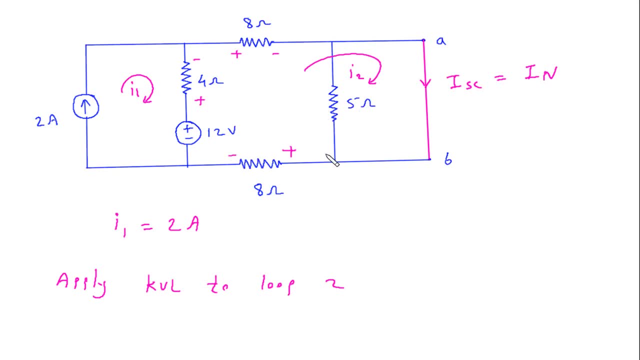 We will ignore this 5 Ohm because it is short circuited. So let's say we will start from here. So this will be plus 8 into I2, then plus 4, plus before, plus 4,, minus 12,, minus 12,. 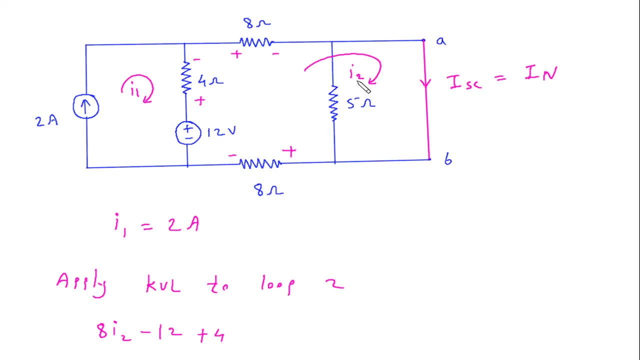 then plus 4, I2 minus I1.. So I2 minus I1 is 2A. then plus 8I2 is equal to 0.. So this will be 8I2 minus 12 plus 4I2 minus 8, plus 8I2 is equal to 0. 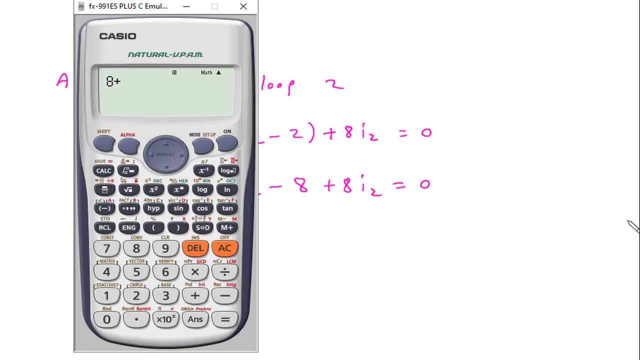 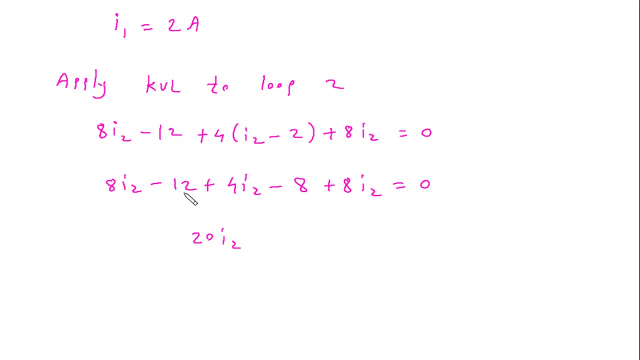 So this will be 8 plus 4I2.. 8 plus 4 plus 8.. So this is 20, 20I2 and this will be minus 12. minus 8 will be minus 20 is equal to 0.. 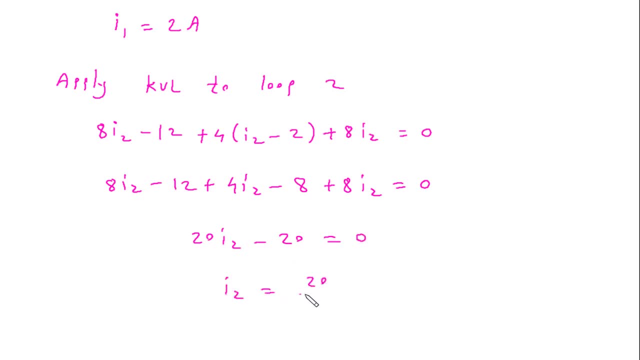 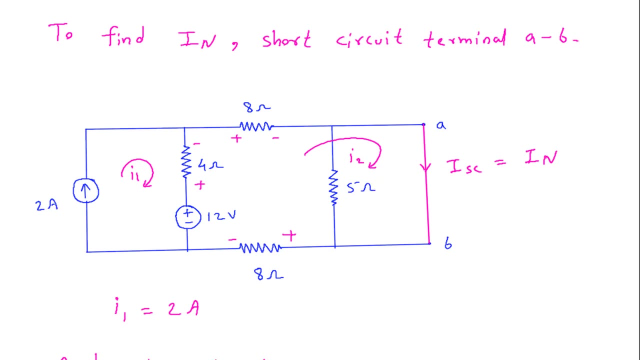 So this will be: I2 is equal to 20 by 20.. So this will be 1 Ampere. I2 is equal to 1 Ampere and I2 is equal to IN, or IN is equal to I2.. Therefore, IN is equal to 1 Ampere.